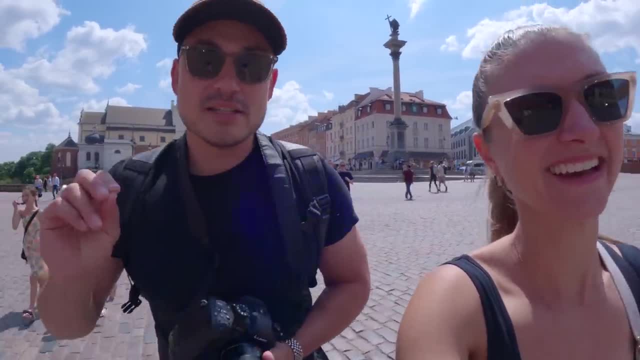 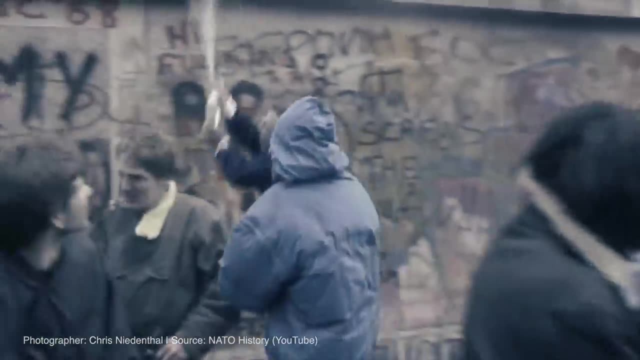 but so far I'm just like: how have I not heard more about this place? We almost skipped Poland, and shame on us for that. As naive foreigners, it's easy to see Poland from a skewed lens and just dwell on the communist era or just focus on the World War II atrocities. But there is so. 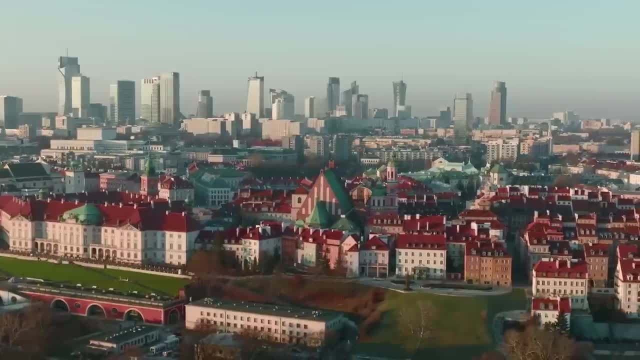 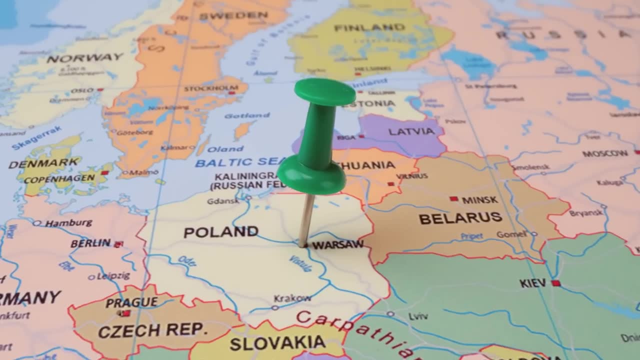 much innovation and growth and beauty in Poland, right now that we had completely overlooked Warsaw. officially, the nation's capital and largest city lies in the heart of east-central Poland, in central Europe, And when I say that this place was bombed during World War II. 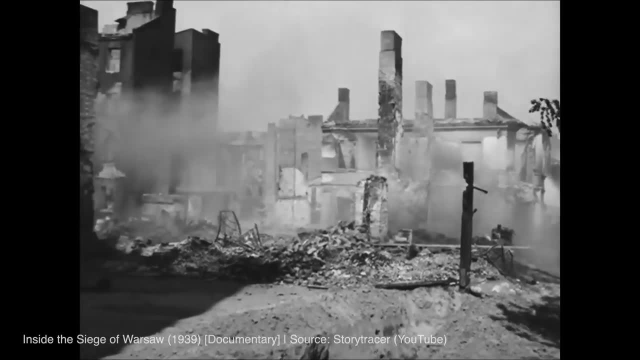 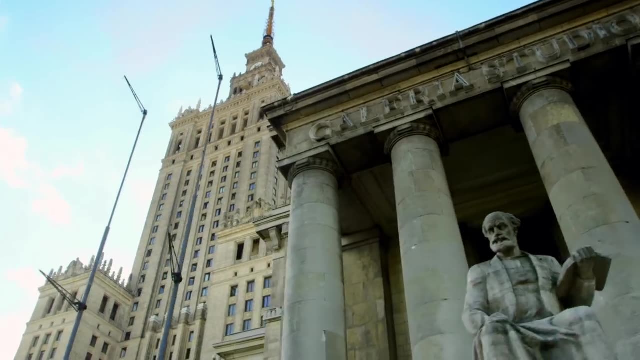 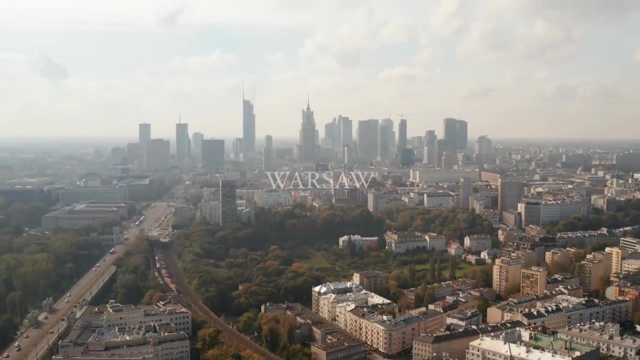 I mean, this place was totally leveled to the ground And looking at the city now, you just wouldn't know it. Seriously, this city has truly risen from the ashes like a baby phoenix. In the past 30 years, Poland has been going through a drastic transformation. 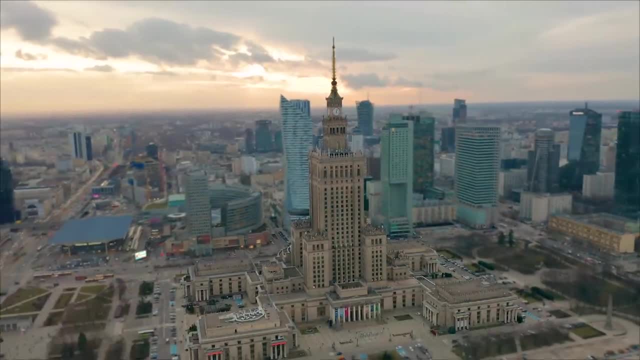 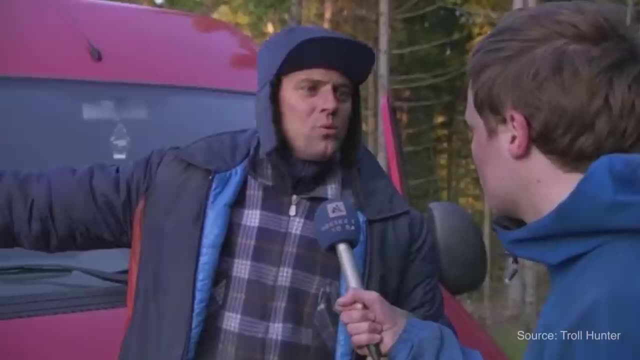 growing more than any other economy in Europe. A recent article came out saying that Poland is projected to overtake the United Kingdom in wealth by 2030.. In Poland we ask, not we do. Why problem make when you know problem have, you don't want to make? 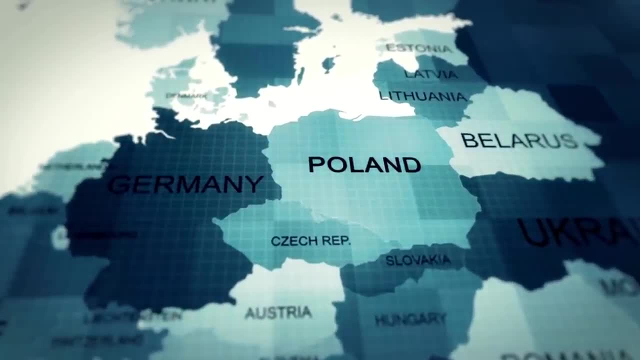 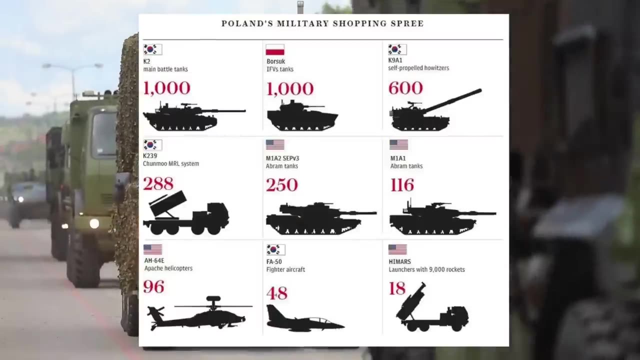 Poland is situated in the middle of Europe's geopolitical frenzy, with Russia, now in Ukraine to the right, Germany to the left. Poland has been investing very heavily in military defense and gaining serious military muscle. I'm talking tanks, jet fighters, Apache helicopters. 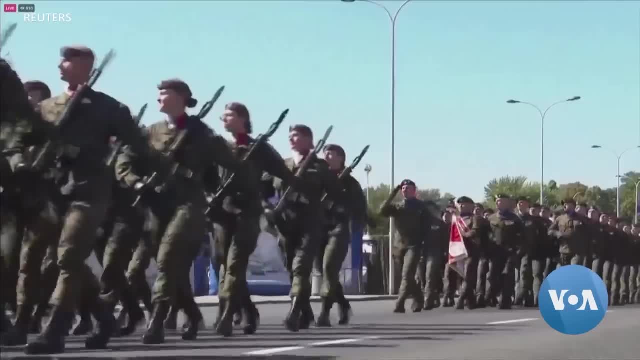 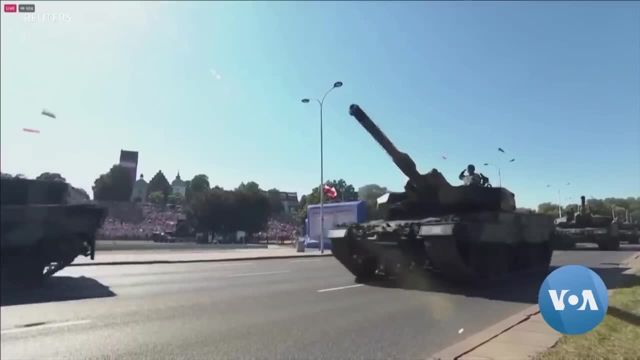 and has doubled its military forces to over 300,000 personnel. Defense is a big sector and all these things cost, So we wondered how is Poland able to finance all this while so much of Europe is going through a recession and struggling financially For one. 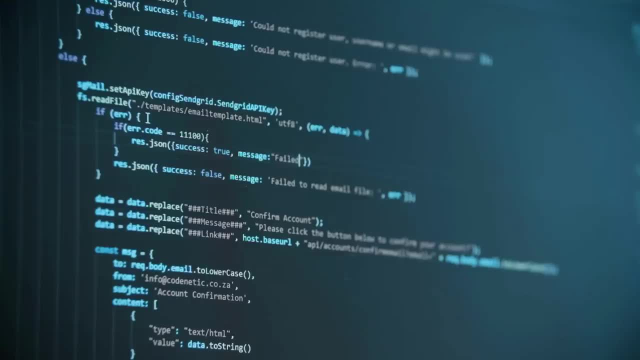 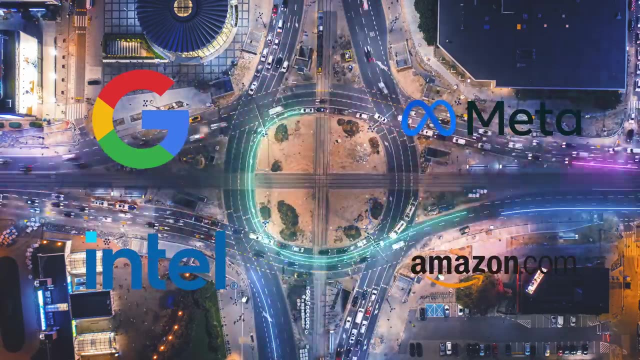 Poland's tech sector is booming and, with a highly skilled workforce, receiving widespread investment from multinational companies like Google, Meta, Intel and Amazon- you might have heard of them- So there's been a huge influx of capital. Much of the world has been sleeping on. 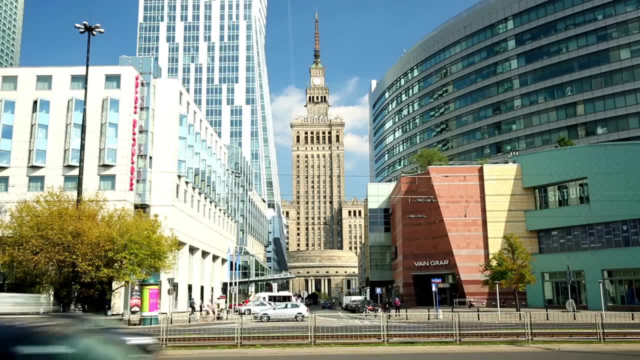 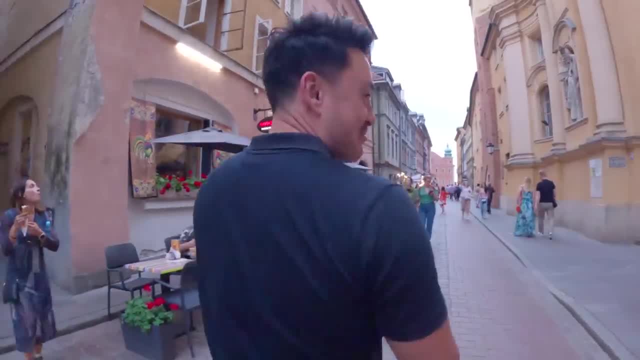 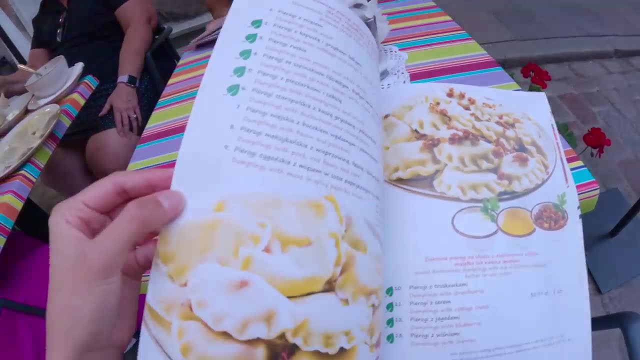 Poland's growth, but more on that later. First, pierogies, You walk so funny. Remember that, pierogi you do. I'm pronouncing it all wrong, Pierogi. Yeah, there you go. That sounds good, All right, this is what we came for. pierogi and pierogi dude, And look at this. 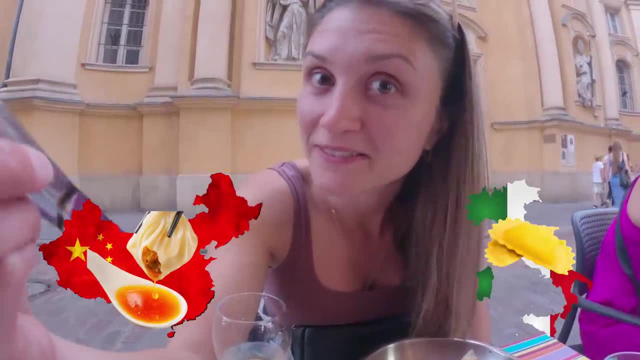 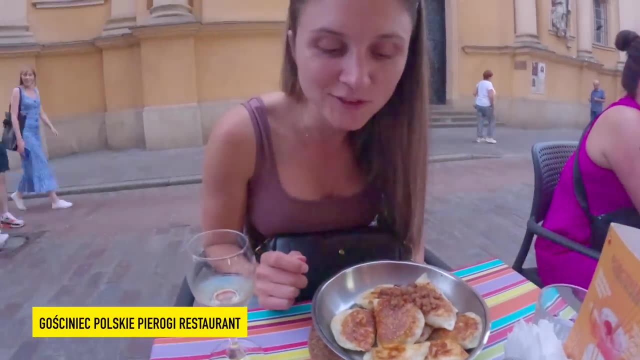 The Chinese got their dumplings, the Italians got their ravioli, but the Polish got their pierogi. That's right, Dude. I didn't expect them to be crispy. I'm down, dude, I'm down. I'm super stoked about that. Listen to this crunch. 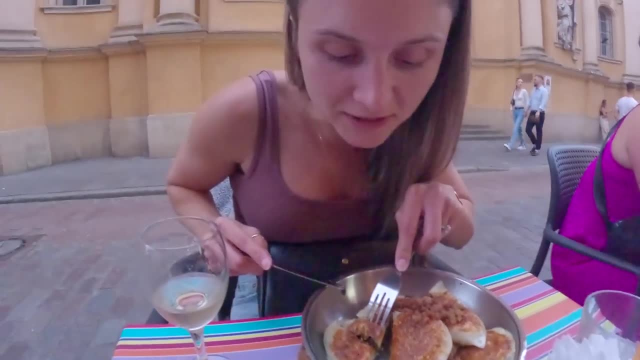 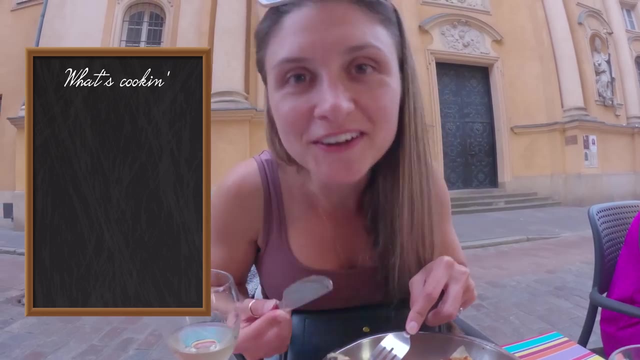 And on top of this is a little bit of bacon. We're doing a little bit of pierogi roulette because we ordered like four different types: A champignon and onion. We got a meat. You say that French too. Champignon- Hey, I tried to say it the right way. We got a meat, We got a. 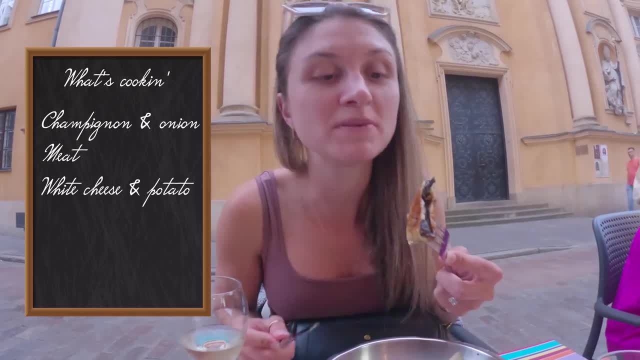 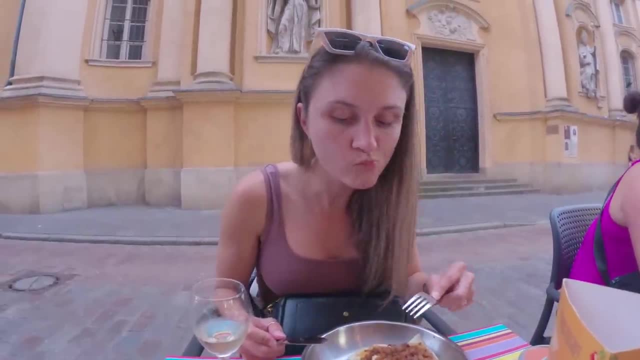 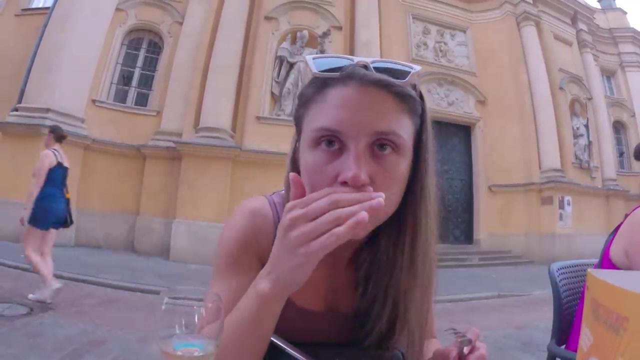 cheese and a white cheese and onion, A white cheese and potato, And potato. So that one already. that's a mushroom for sure. Yes, this one's a champignon. Okay, that's right, It's quite hot, Oh my God, Oh my God, Holy shit, This is better than any dumpling or ravioli I've ever had. 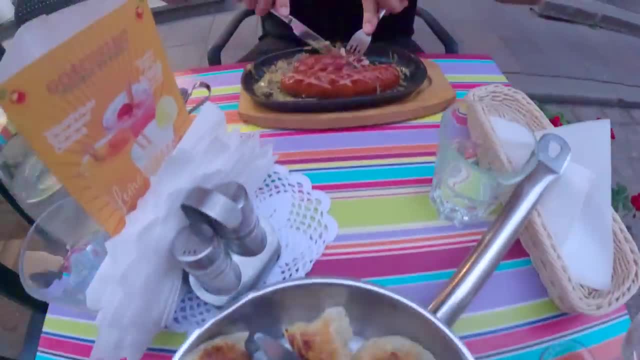 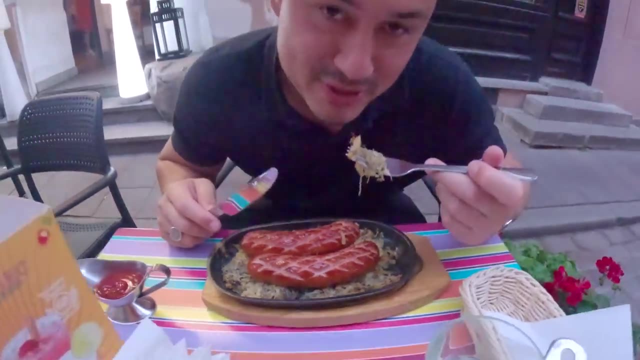 I'm not saying that for the clout. This place, this place has like phenomenal reviews. We got ourselves a Polish sausage on top of some sauerkraut- One of my favorite things in the world. I love sauerkraut. That acid with a fatty meat- Oh my God, Dude, it looks amazing. You hear that. 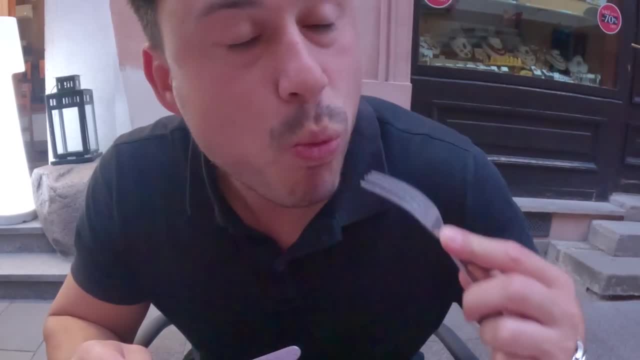 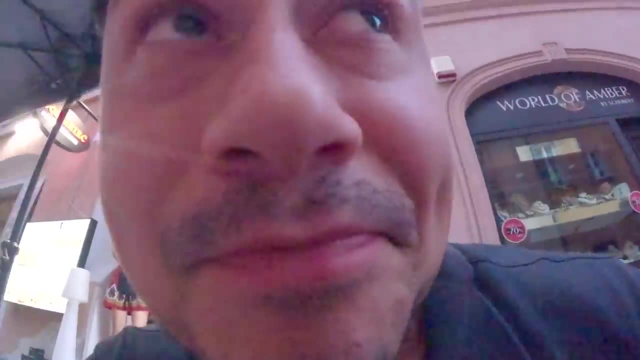 The outside skin. That's what you want. You want that snap, Wow. All right, we'll be back tomorrow. All right, we back Round two. Pierogies, round two. Boiled is like the more traditional way, although a lot of the locals 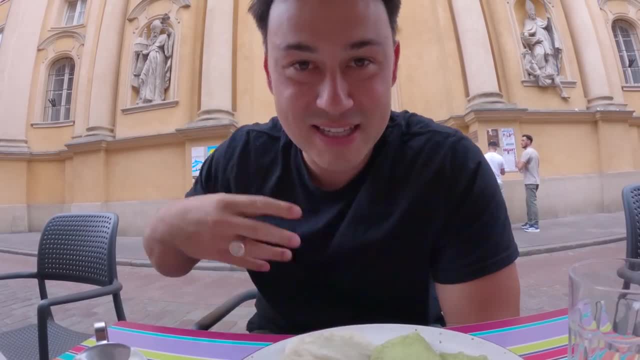 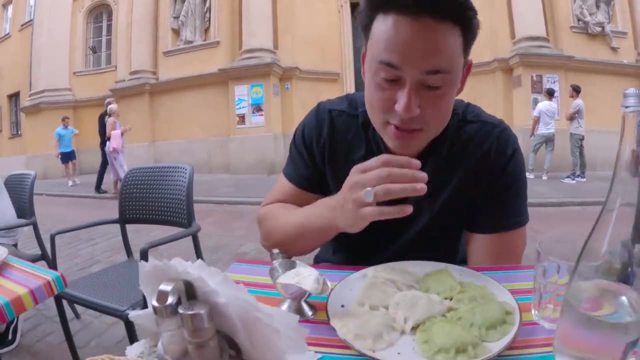 prefer it fried, because obviously anything fried is typically better. You got like texture, you know, kind of crispy on the outside. Oh yeah, A little side of sour cream to compliment that. Instead of the bacon, Instead of the bacon. Yeah, this is a little bit. this is like the. 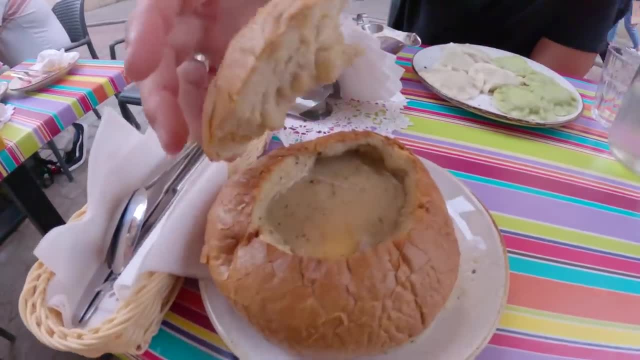 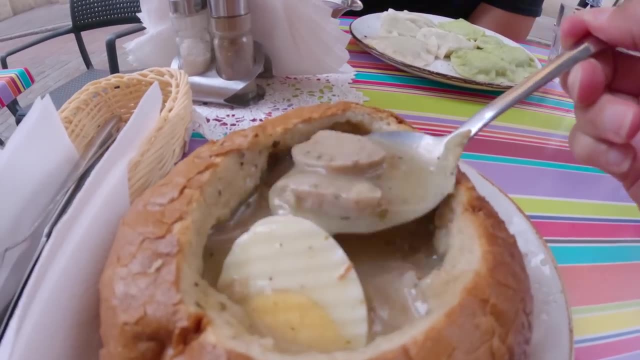 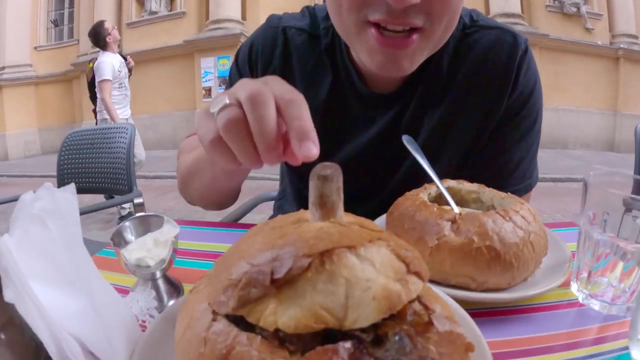 healthier version. basically, Sorry, I'm so, so busy. Soup, That's like a sour rice soup, served in bread with like white sausage egg, all kinds of goodness. This is an old Polish hunter style pork stew. It looks like a little hut. Okay, It looks like a little house with a chimney. It's so cute. And if 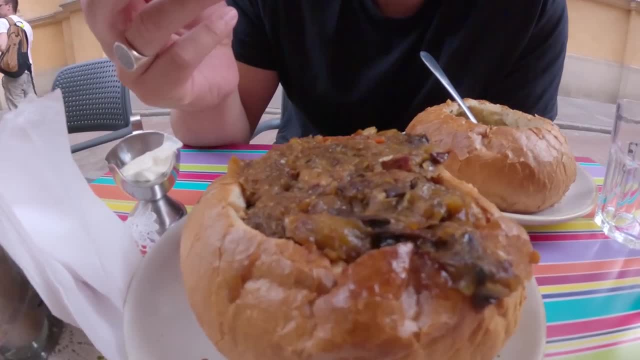 you open it up. look at that. I don't even know. I heard there's plums in it. It looks like there's like a sauerkraut in it. It's obviously got some pork in it, but please dig in. It smells amazing. 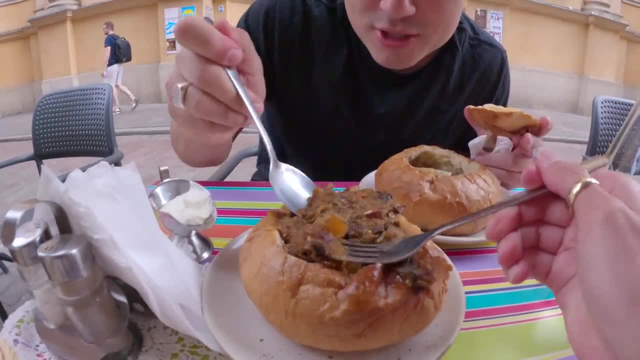 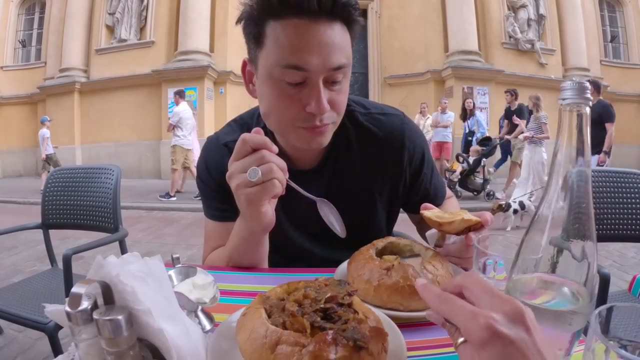 Oh my God, Can I just dig in? Can we both dig in? Let's do it. There's no rules, right? Oh my God, They're both really good. I love how sour this one is. It really does taste like. sauerkraut. Yeah, And this one's got the sweetness from like that fruit. It's got a little bit of sourness to it. It's got a little bit of sourness to it. It's got a little bit of sourness to it. 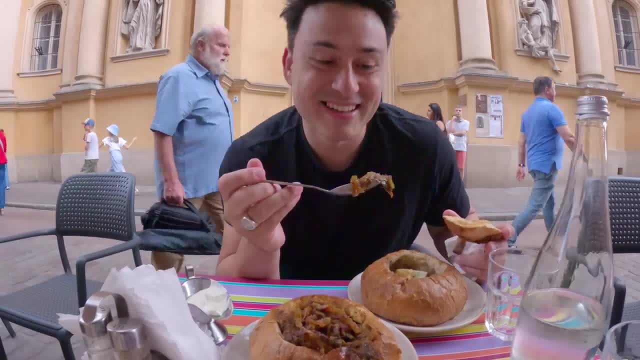 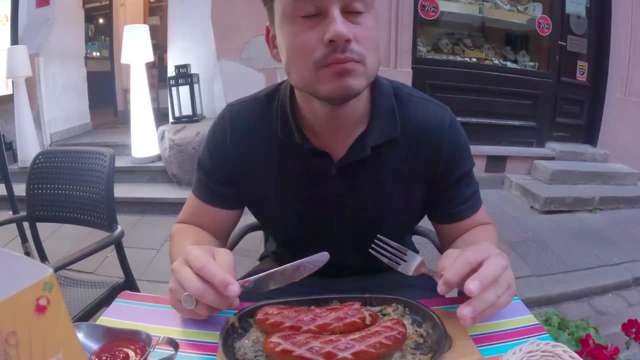 And this one's got the sweetness from. like that, fruit Delicious, And after a hearty meal like that, and, dare I say, pierogi heaven. you know we need a nap And that's where today's sponsor comes in: Brooklyn Bedding Traveling. 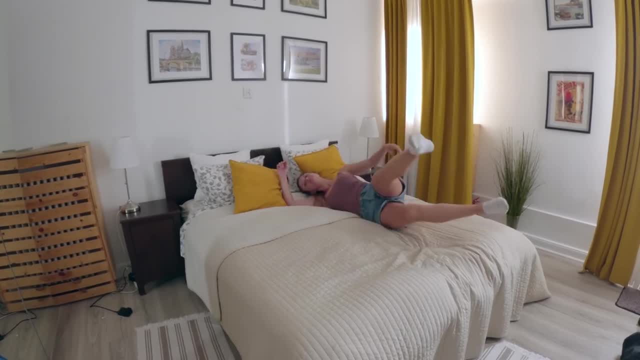 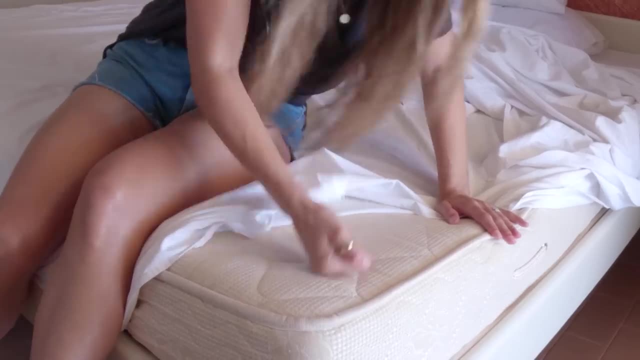 full-time means we don't always have a say in the quality of the mattresses we sleep on. They rank from bad, decent, good to pretty awful. There's no gift in this mattress, But if we had the option or could teleport to our mattress back home. 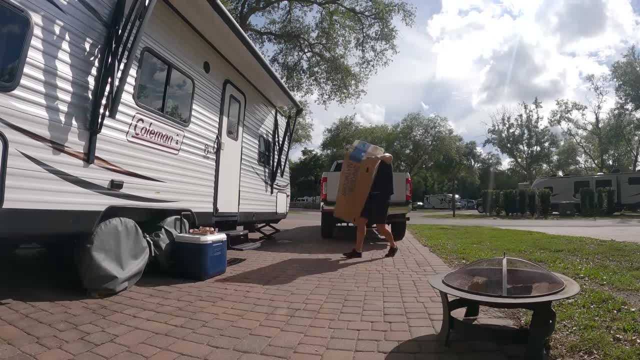 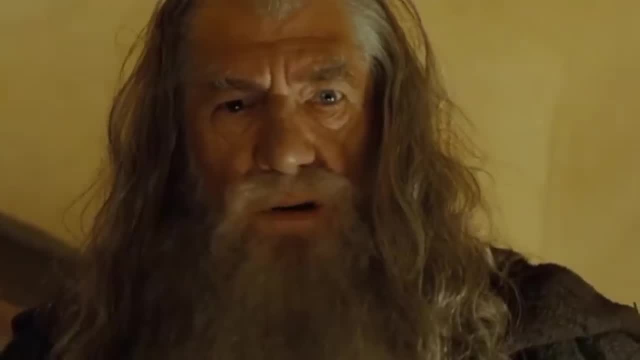 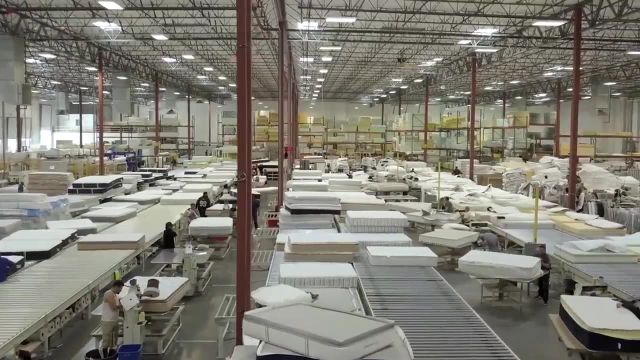 we'd choose a Brooklyn Bedding mattress all day long, Our personal choice of bed to rule them all, My precious Precious Brooklyn Bedding offers a wide selection of sizes and firmness levels to best suit you, And they own their own factory in the US, which allows them to offer super high quality mattresses. 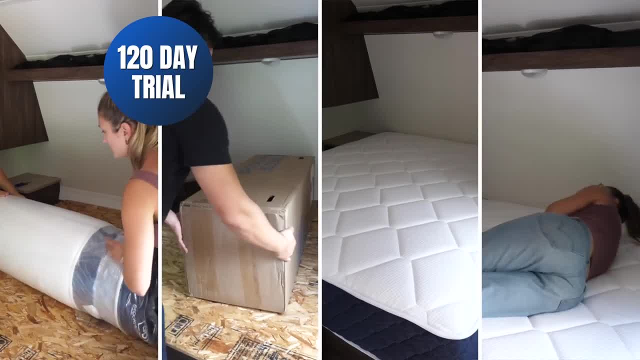 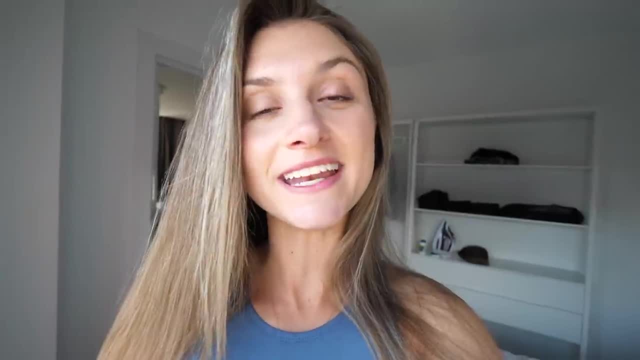 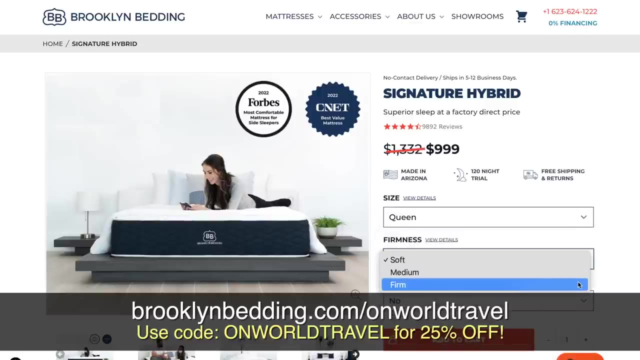 without the luxury price tag. They offer 120 night sleep trial, free shipping and a 10 year warranty. So if you want to upgrade your mattress, just like we did, head on over to brooklynbeddingcom onworldtravel and use our code onworldtravel to get 25% off. 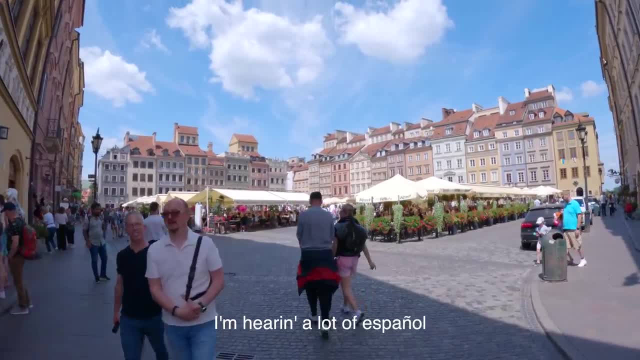 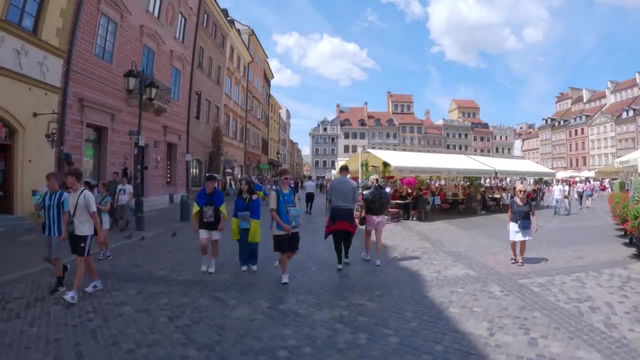 What is popping? I'm hearing a lot of espanos. Yeah, What is going on? There's a lot of- The spaniards are taking over Warsaw. Yeah, Yeah, Good energy though I'll say. And all these… the facades of the old town are-. Really well intact, Yeah, Well-maintained Or I don't know. They usually took things for a while. I wouldn't say anybody was dirty… But lol, it wasn't really like high end or anything. Really, Really. 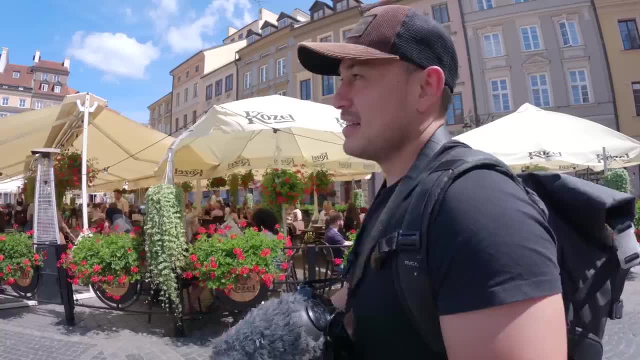 Yeah, Yeah, Yeah. I really wouldn't buy this mattress. Well, I的 don't know. They usually touch them up every few years, but this is one of the nicest ones. Is that what they do? They touch them up, They touch them up, You know, just a little bit Dab dab here and 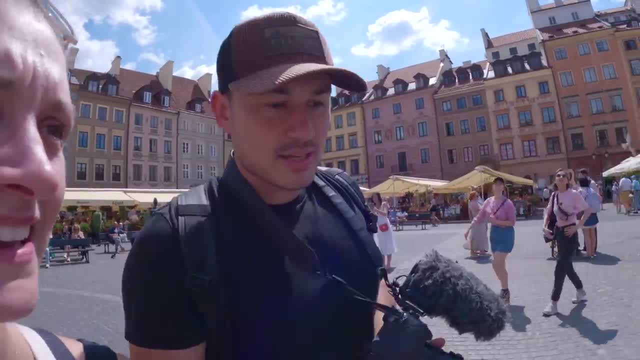 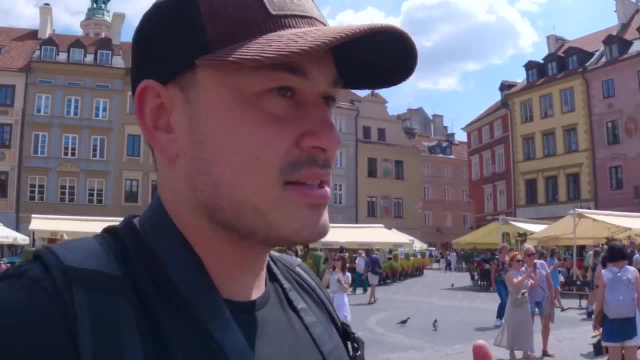 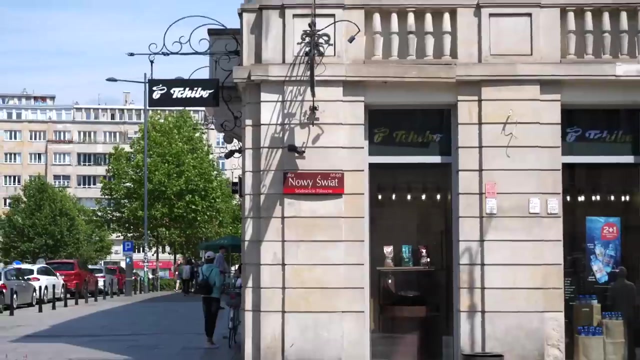 there, Patch up the holes. They have the butt cheeks right in the center of the square, right there. That's what you want. That's what brings it all together. The cohesiveness of the square is the butt cheeks. All right, we're now walking down. Novi Sviat, Sviat, Novi Sviat, Novi Sviat. 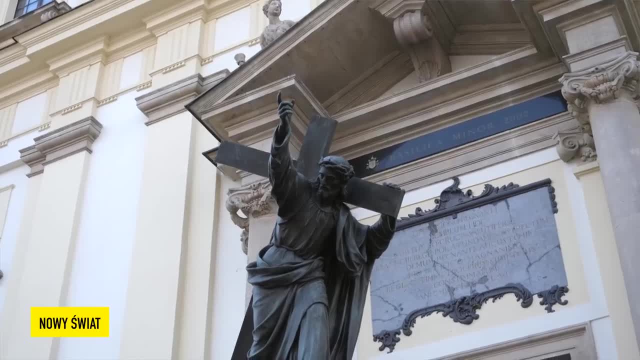 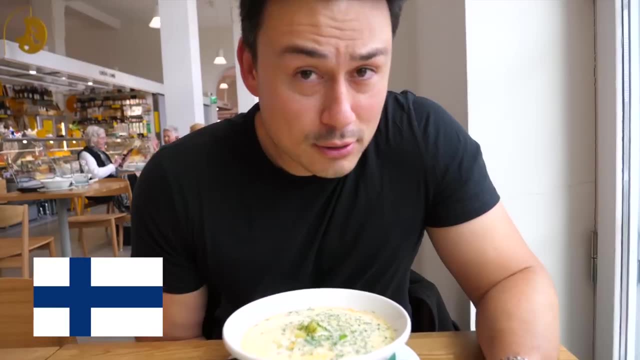 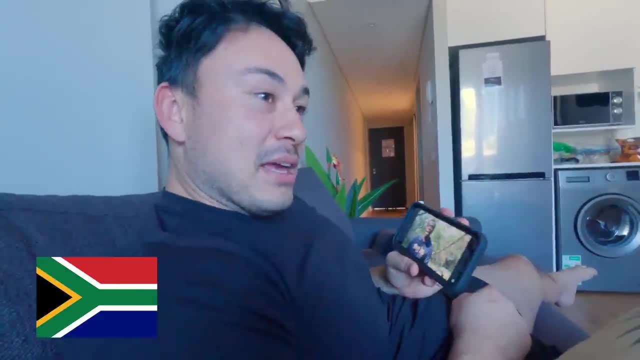 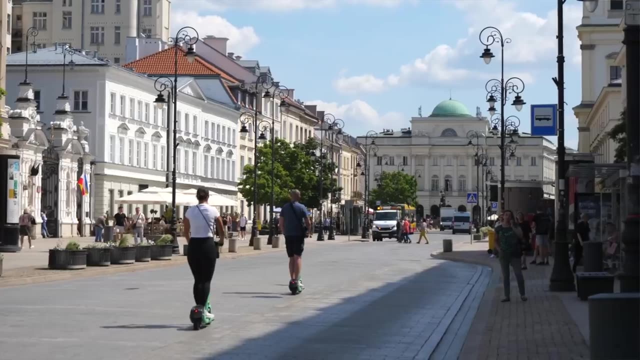 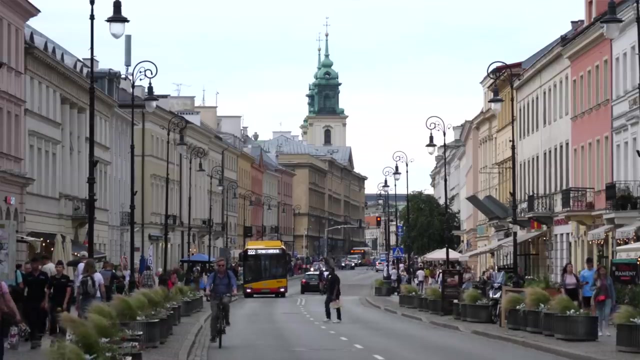 I feel like this street like based on what I've read online- is kind of like the Champs-Elysees type of Warsaw. There's like a lot of restaurants, a lot of cafes, a lot of shopping, It's busy, it's people are out and about, it's popular and, yeah, it's also very charming, just the different. 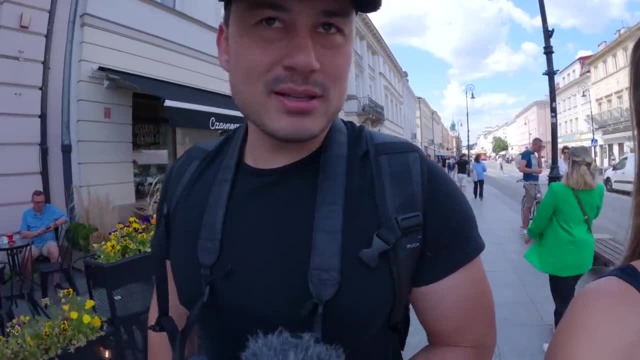 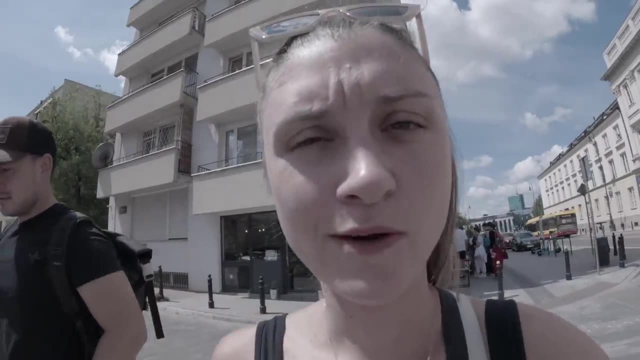 colors of the buildings, different architecture. But, uh, we're gonna grab another cup of coffee because we gotta make up for that one we had this morning. Yeah, Thank you. Thanks so much. All right, well, that way was the most watered down, milky, flat, white. I've ever had in my life. I'm taking no prisoners. I'm going only 4.5 stars and up. Look at the photos. Like. that's not for me. I mean, maybe I'm a little bit of a coffee snob. 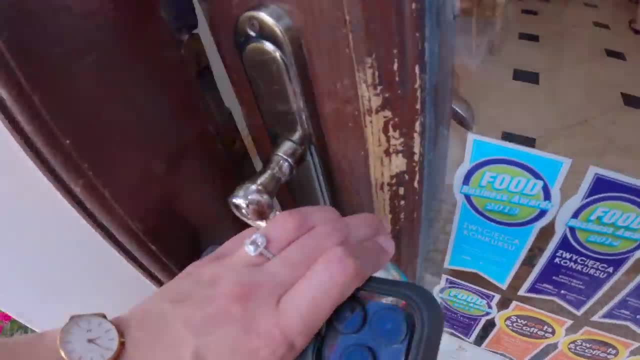 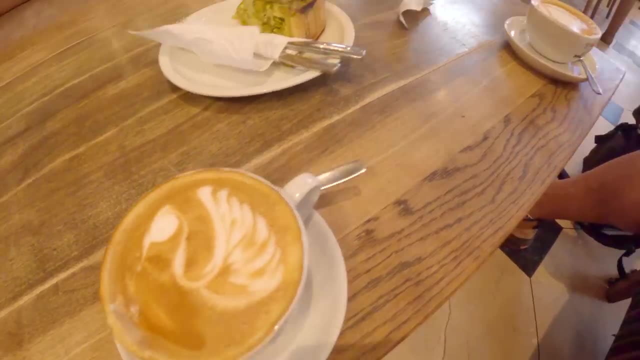 That's not a good cappuccino or flat white. It's really nice. Oh, if you just want a good flat white, I'm telling you: Like, look, and they can do the design. and just like, not too much milk. 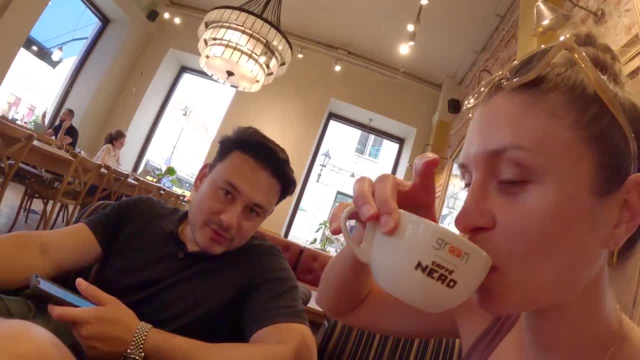 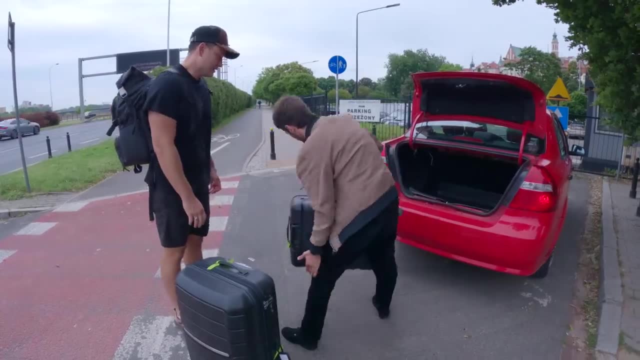 Like it's a proper flat white. They do it really good here. Usually I'm not one for flat whites. I like them voluptuous whites and curvilicious whites. Nathan, you're psychotic. The food bag You brought the peanut butter. 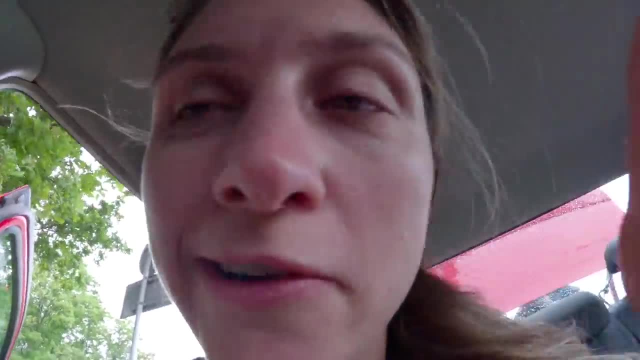 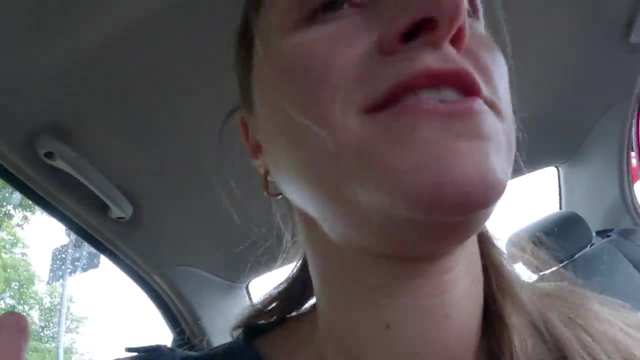 Yeah, I did, Dude, it was one bite. Nathan always got priority. You know what I'm saying. We gotta keep a olive oil and balsamic and eggs and all the other weird shit we do. All right, first flex. 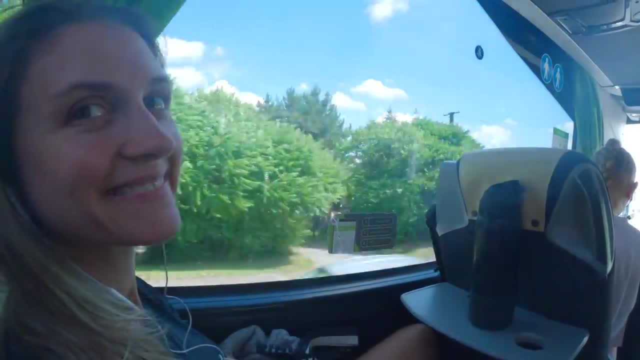 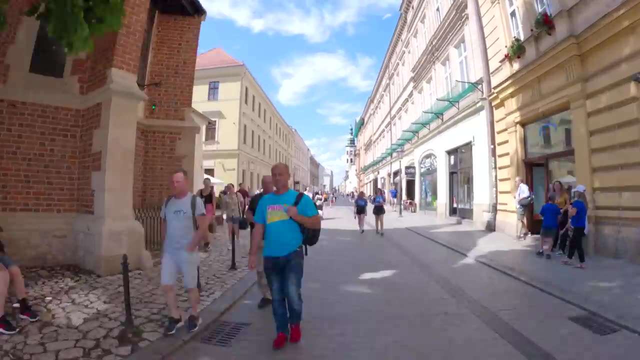 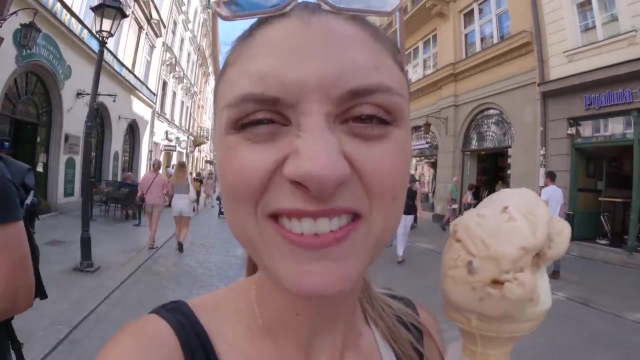 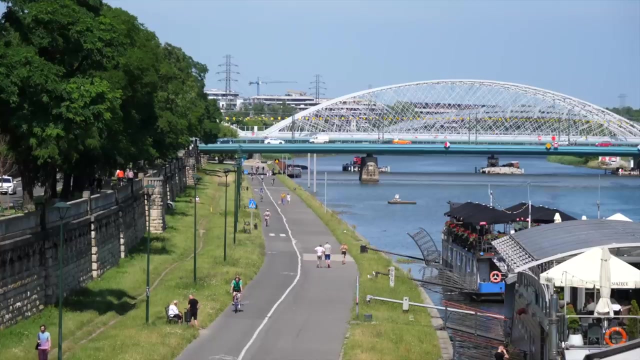 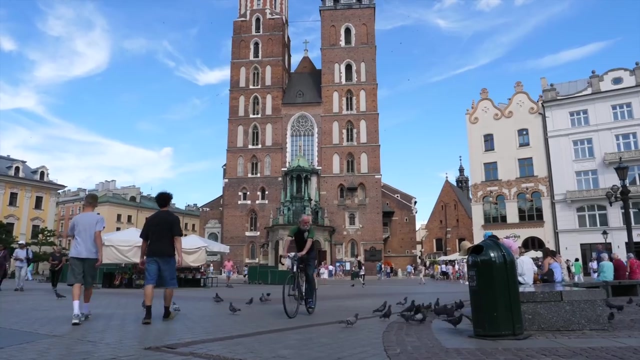 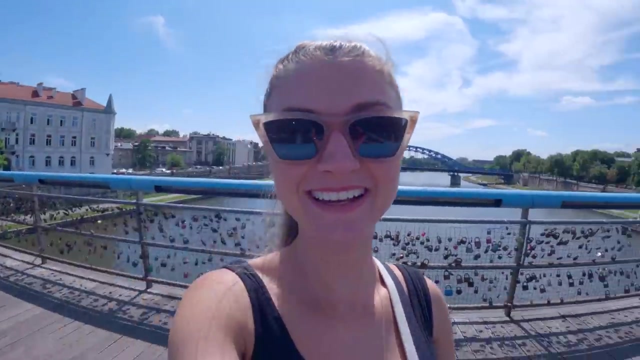 Another day, another bus, Dude, this is nice. What's going on with Poland? I don't know. I don't know, I don't know. All right, so now we have a couple days here in Krakow. A lot of the locals here, they told us. 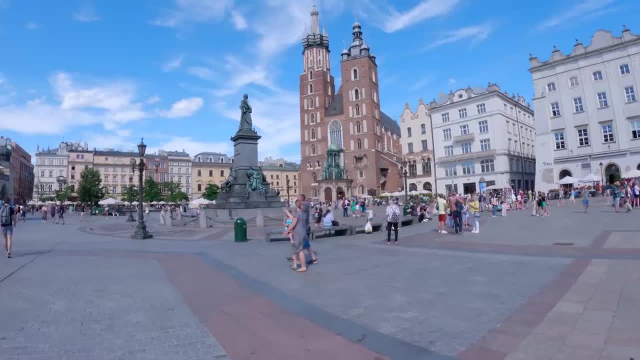 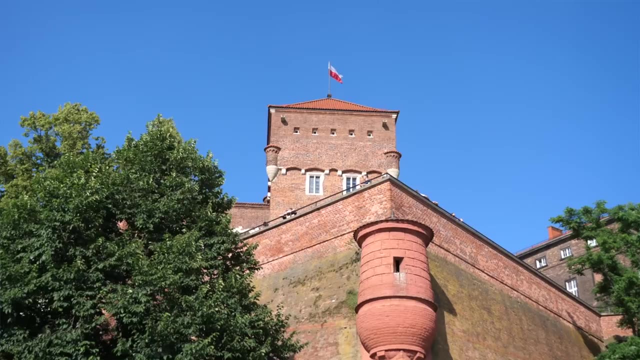 that if we have limited time in Poland, which we do, we're here for just over a week. they recommended that we actually spend more time in Krakow, over Warsaw, and or if we can make it to Gdansk. We're not gonna be able to make it to Gdansk. 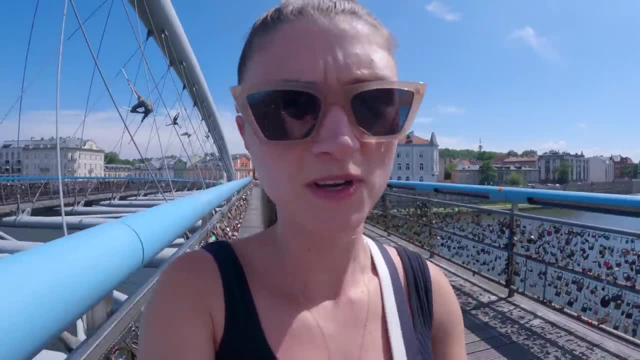 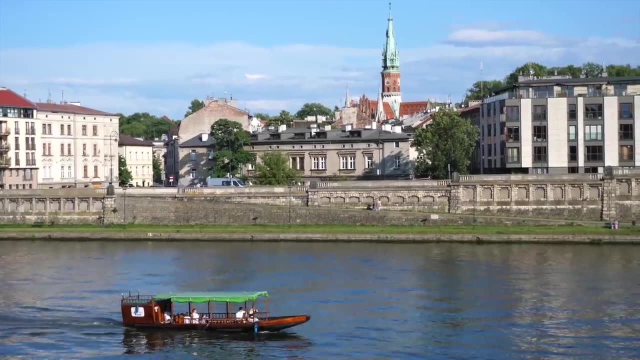 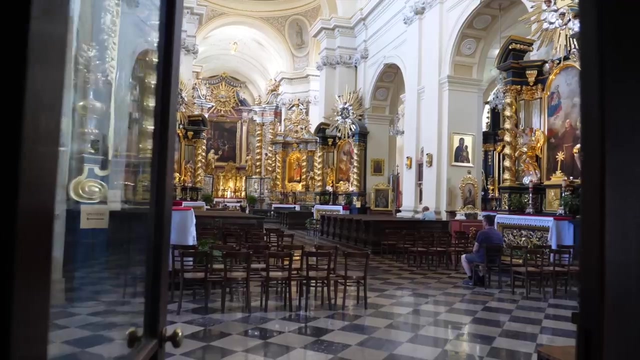 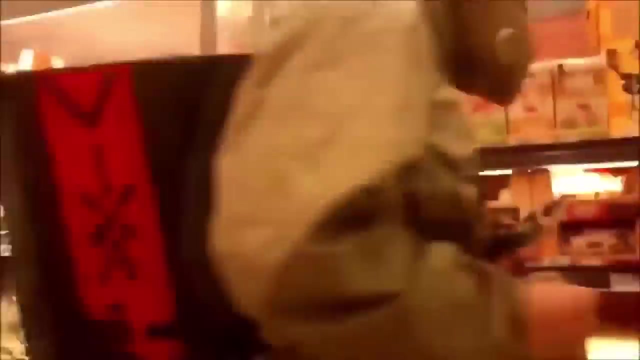 I hope I'm saying that right. LOL, I'm gonna look back at this and be like what the? But so far, Krakow has a totally different vibe from Warsaw. Haha, Another old town. here we come. Well, we found the Big Ben of Poland. 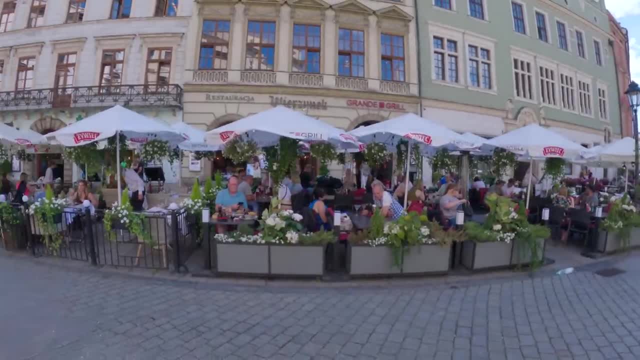 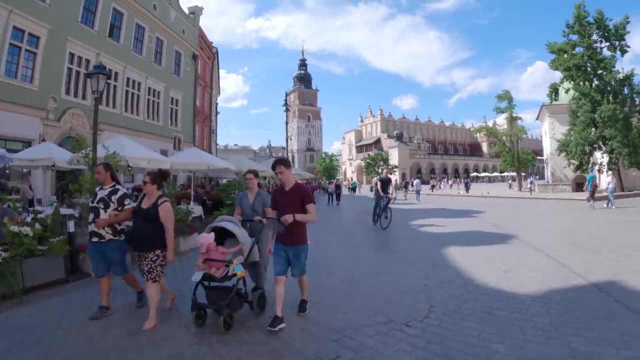 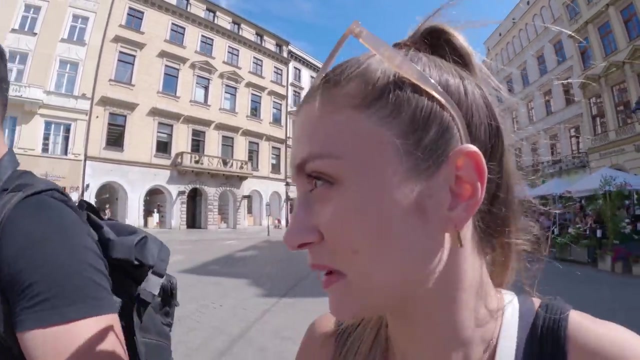 It looks like that totally Outdoor seating. once again, Lots of greenery — cocktails, ice cream, hamburgers. it's a vibe. summer is summer is here for sure. yes and again, i just feel, like the people who live in places, that it gets like really freaking cold, like minus 20 celsius in the winter. we've 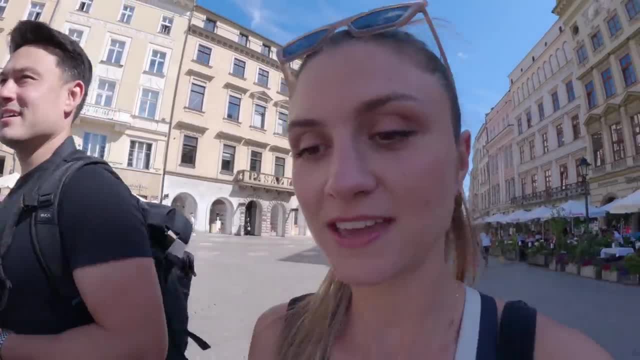 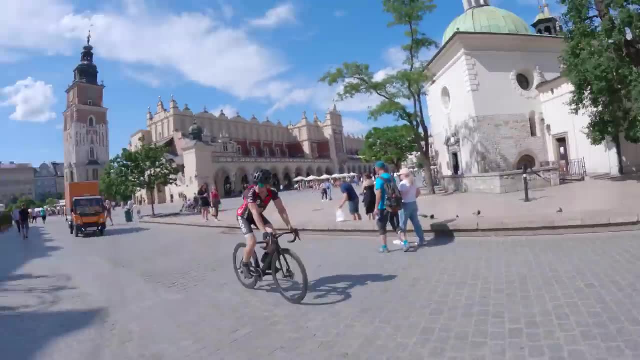 been told they appreciate, they appreciate summer and they actually, yeah, they want to run a bike, they want to get on their scooter, they want to go for walks and, i swear to god, ice cream. look at this guy right here. he is cold, he's cold. okay, dude, he's smacking. this is the life. 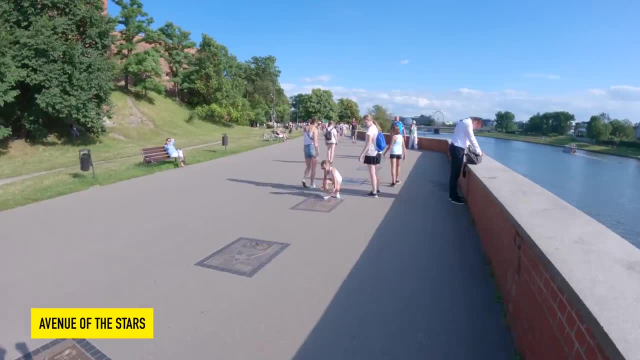 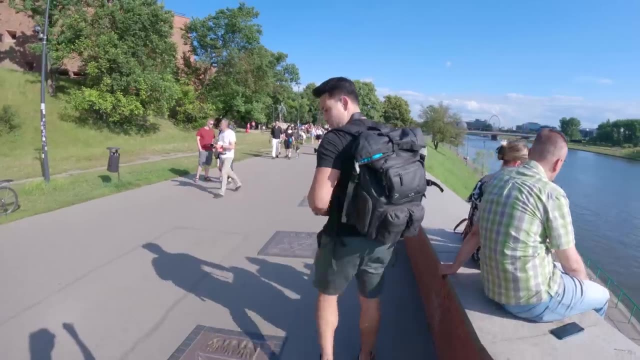 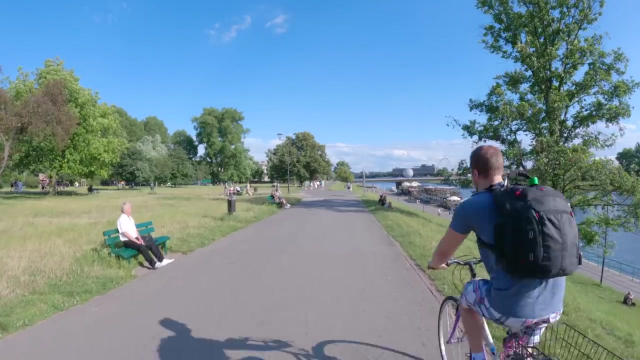 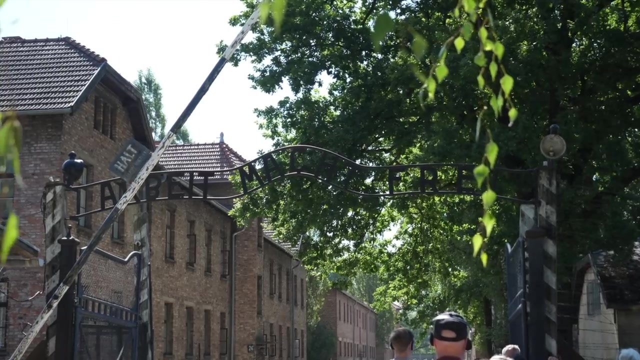 the hands don't fit. you must have quit. stop got that little version of hollywood over here. oh my god, two experiences we included in our time here in krakow. two experiences we included in our time here in krakow. we're visiting the auschwitz concentration camps and the veliksa salt mine. we found an 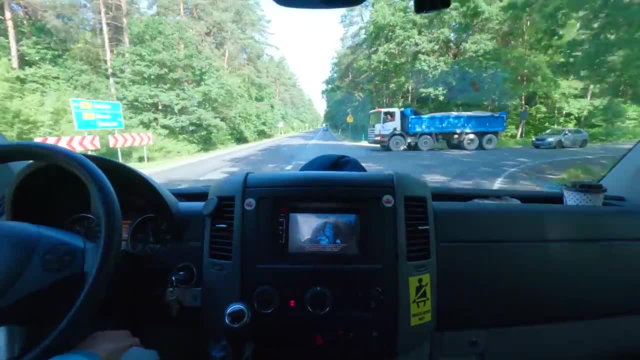 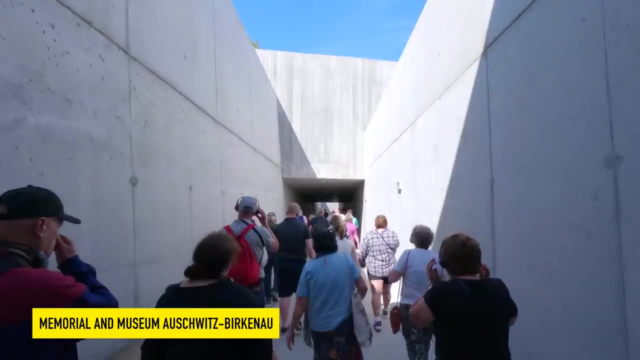 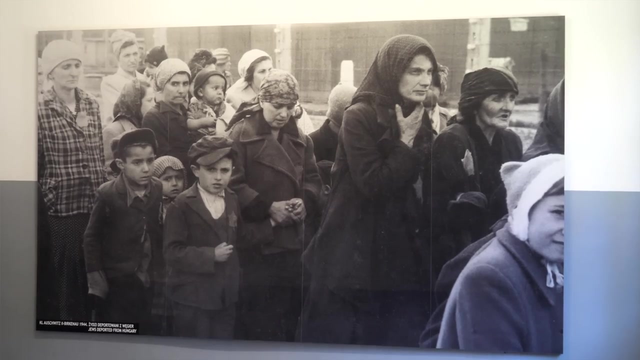 all-day tour that took us to both sites. as heavy as it is, i recommend that every person visit auschwitz. it's an invaluable part of history that is a reminder of what mankind is capable of in the worst sense. one of the first quotes you see is george santayana saying: those who don't. 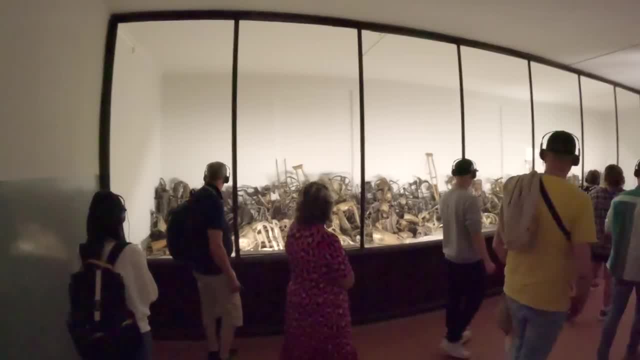 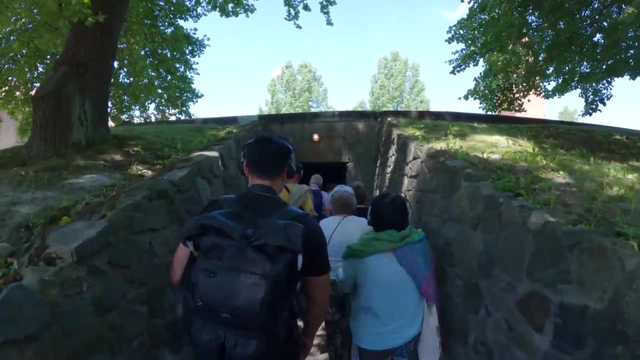 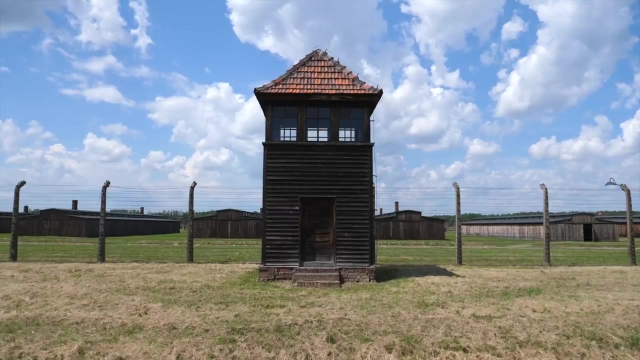 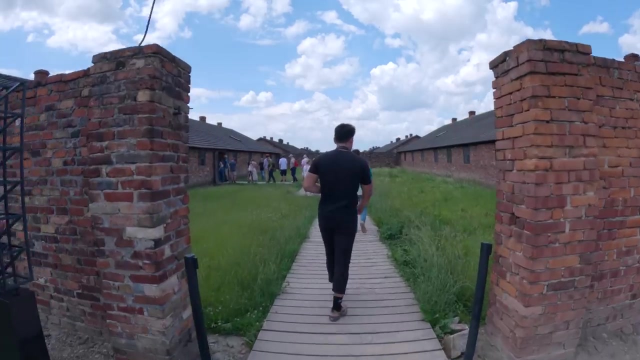 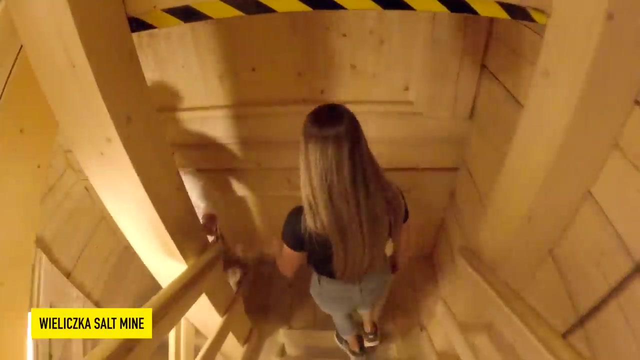 remember the past are condemned to repeat it. the tour guides provide enormous insight into the atrocities that happened here, and it's definitely eerie to be standing on the actual sites of where it all happened now. the salt mine was one of the coolest things we've ever done. we were taken 442 feet underground. 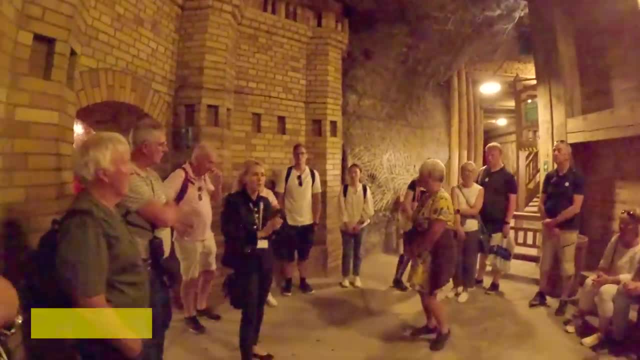 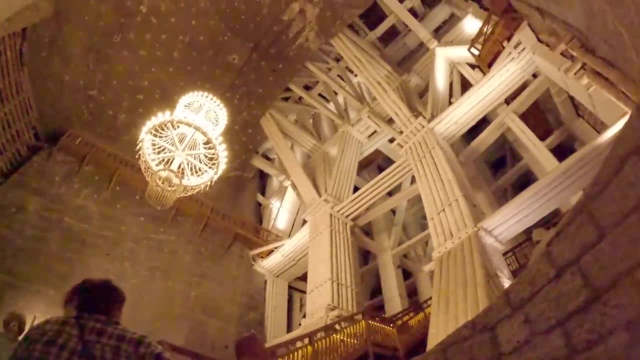 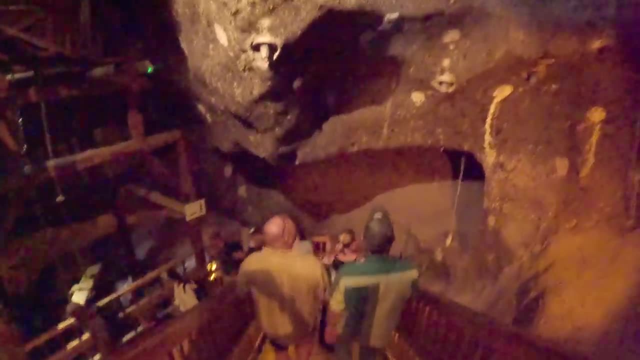 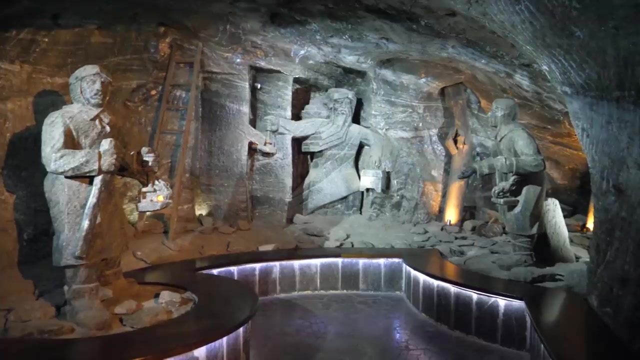 this one connect the first level with the third one. in the past it was also used. we are so like far down right now, claustrophobia. the mine reaches a depth of 1073 feet and extends over 178 miles. since the 13th century, brine welling up to the surface had been collected and processed for its. 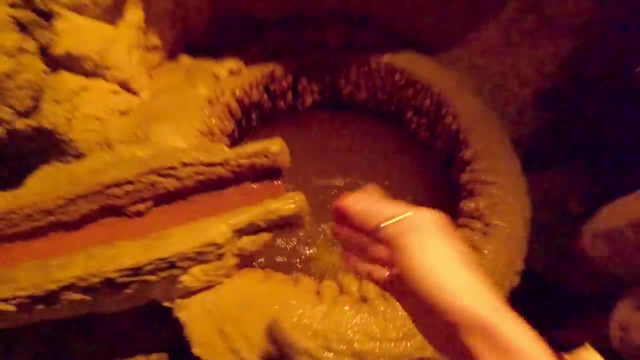 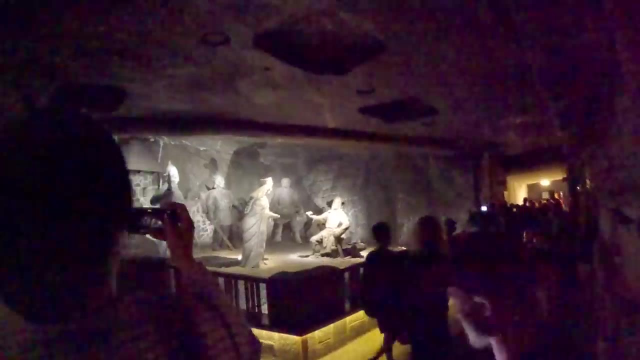 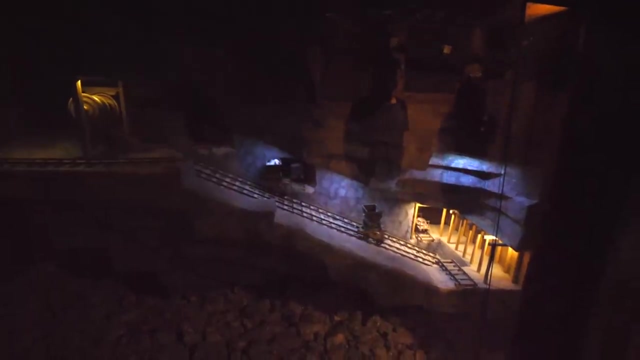 use as a source of sodium chloride content, aka table salt. oh, i got a lot super salty that's saltier than the ocean. today it's home to the krakow saltworks museum. the tour shows visitors in underground lake exhibits on the history of salt mining. 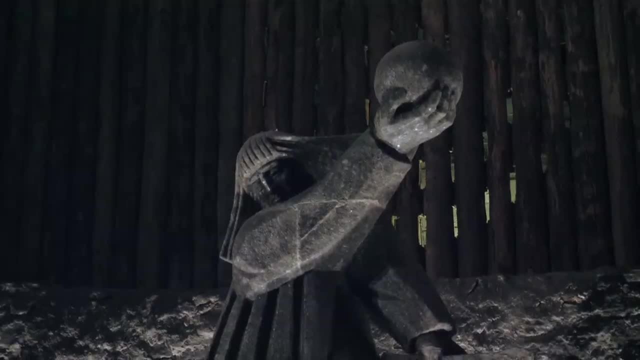 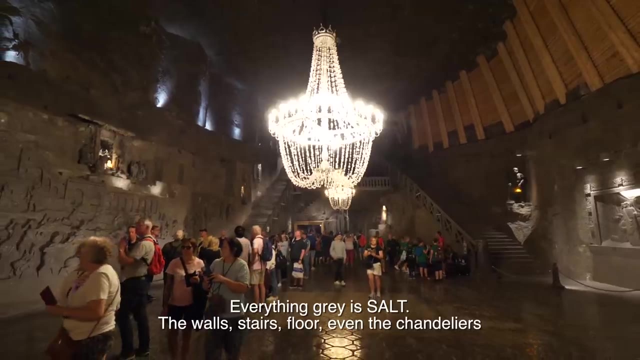 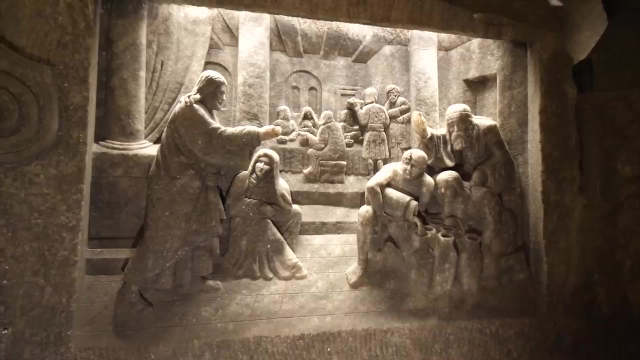 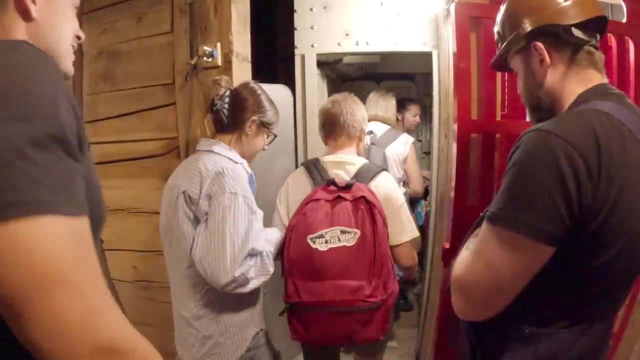 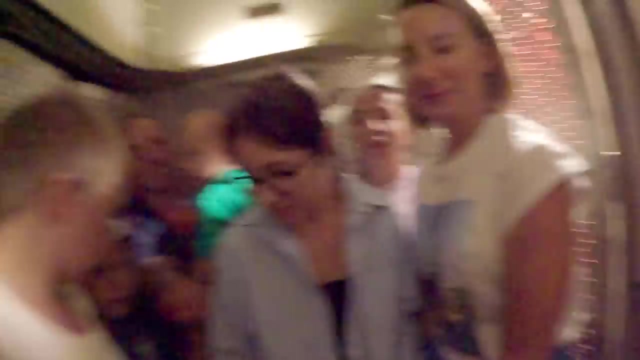 numerous statues carved by miners out of rock salt, but the craziest thing to us was this underground chapel. everything's made out of salt, even the chandeliers. this is so crazy. oh, it's racing. oh it's bigger, it opens up, thank you. oh my god, they are actually.